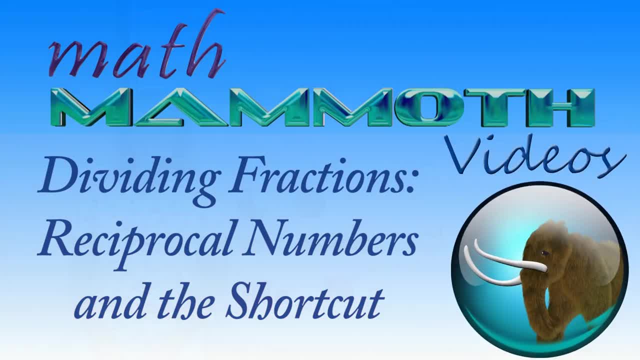 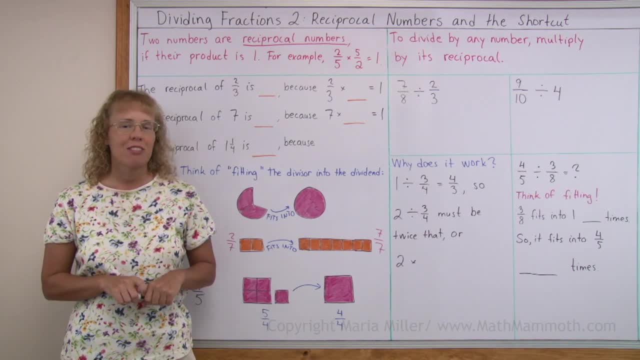 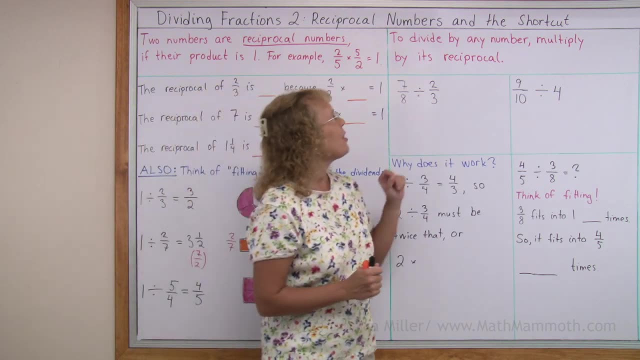 Hello, my name is Maria from MathMammothcom. In this lesson we are studying reciprocal numbers and the shortcut for dividing fractions, which is- it's written over here- to divide by any number, to divide by a fraction or whatever you can multiply by that number's. 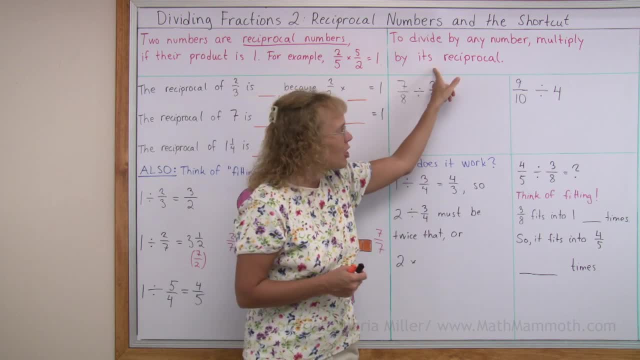 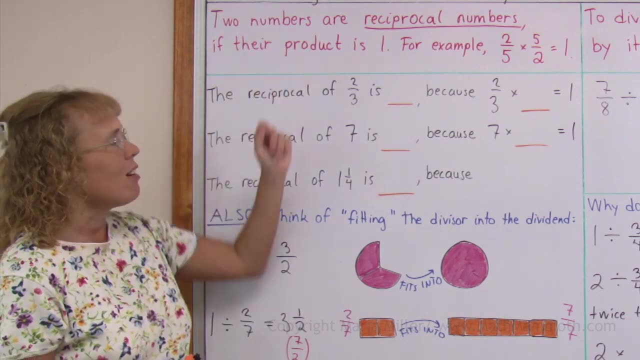 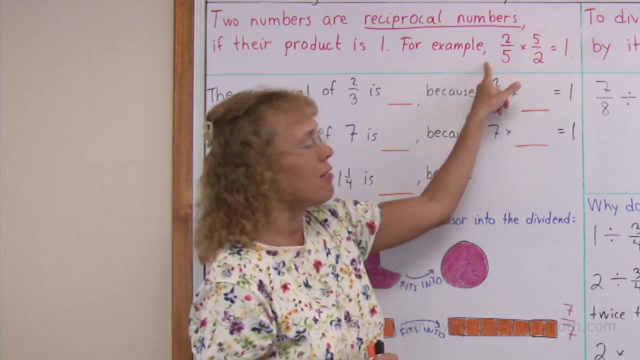 reciprocal. So before we study this shortcut, we need to study reciprocal numbers first. Now, what are reciprocal numbers? Two numbers are reciprocal numbers if their product is one. If you multiply them, you get one. For example, two-fifths and five-halves. 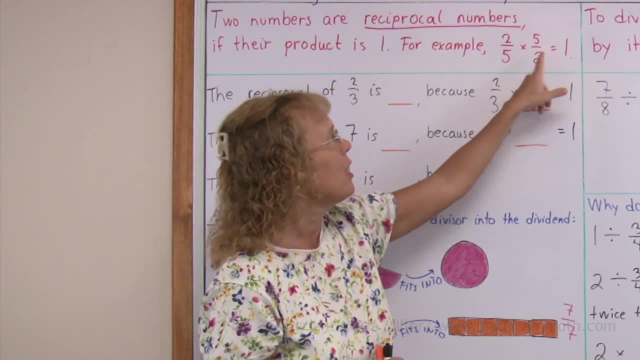 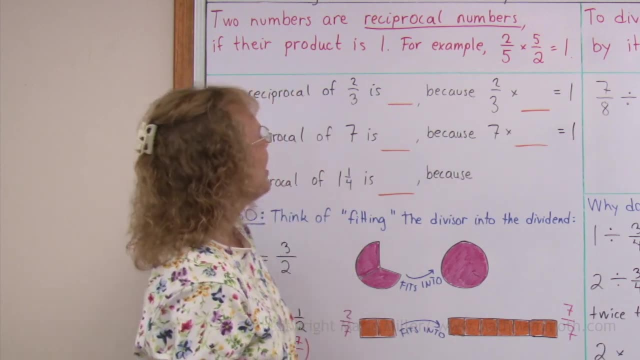 are reciprocal numbers because if you multiply them you get one. You get two times five, which is ten, and five times two, which is ten. Ten divided by ten equals one. Let's look at some more examples. The reciprocal of two-thirds is one. 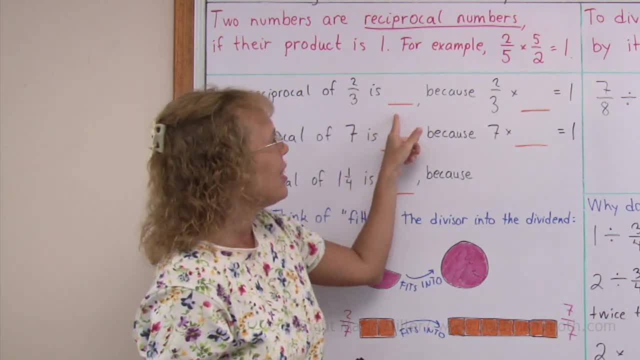 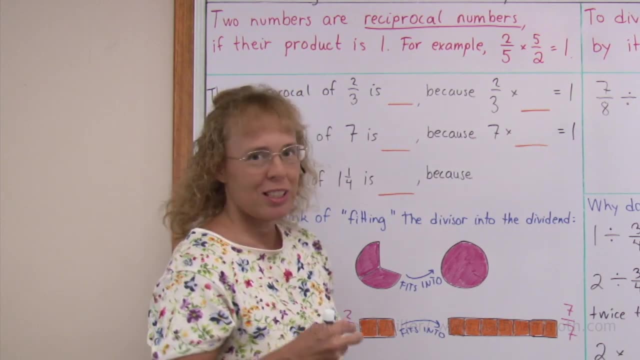 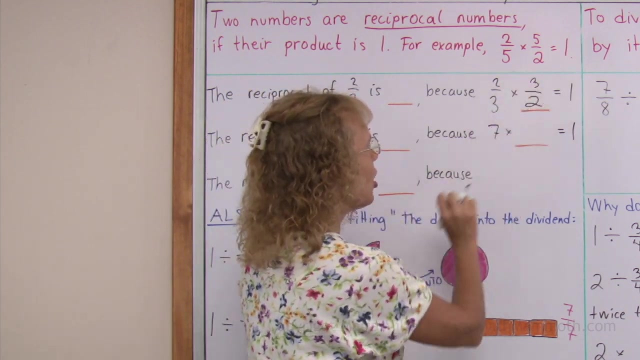 What would it be? It's some number, so that two-thirds times that number equals one. And what we can do is we can flip the fraction. I can write here three over two, because then in the multiplication I get six on top, six on bottom, six-sixths, which equals one. Okay, 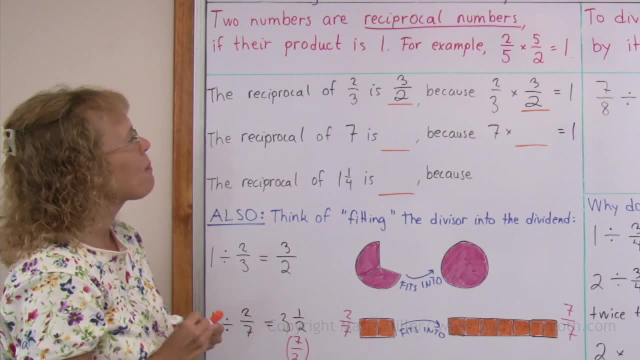 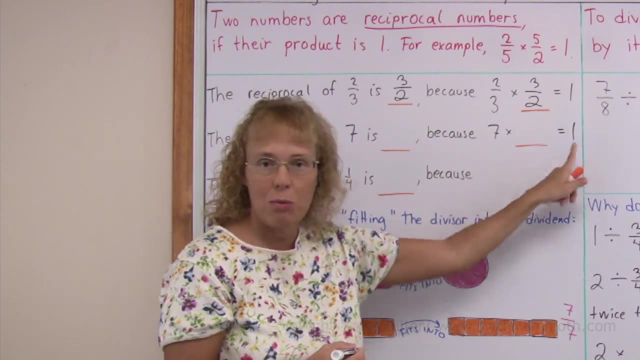 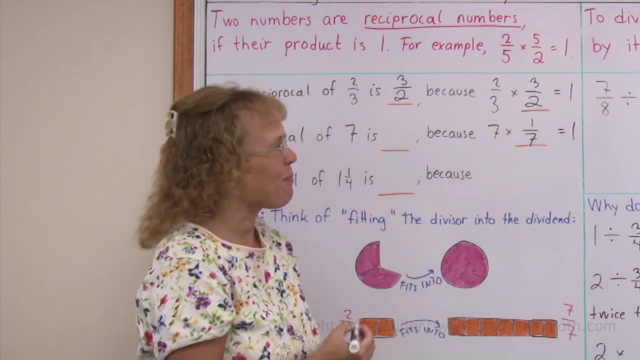 So three-halves was the reciprocal of two-thirds, Then the reciprocal of seven. Think about this multiplication here: Seven times what equals one. You can probably see that seven times one-seventh, right, So over here there's a flipping two. If you think of this as seven over one, then this: 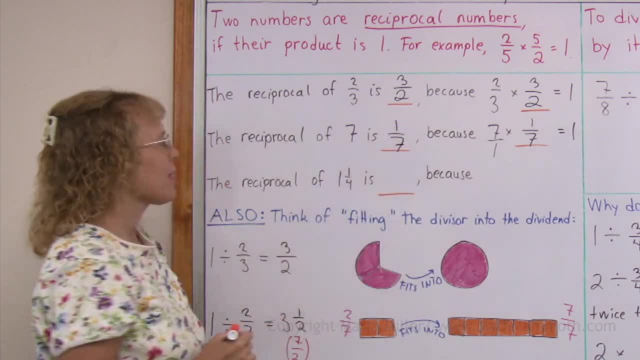 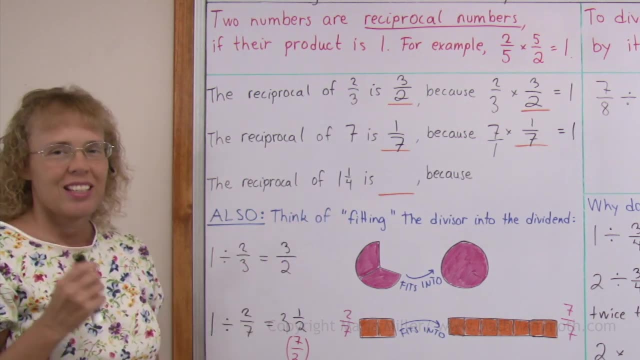 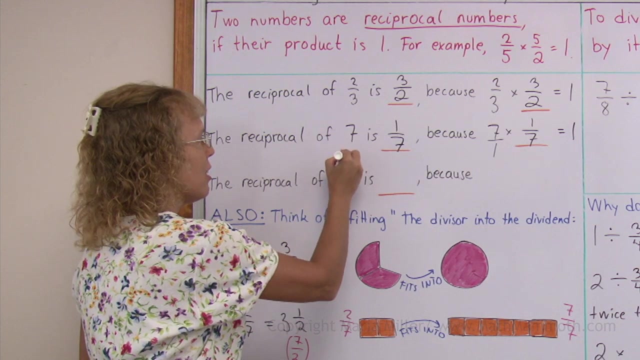 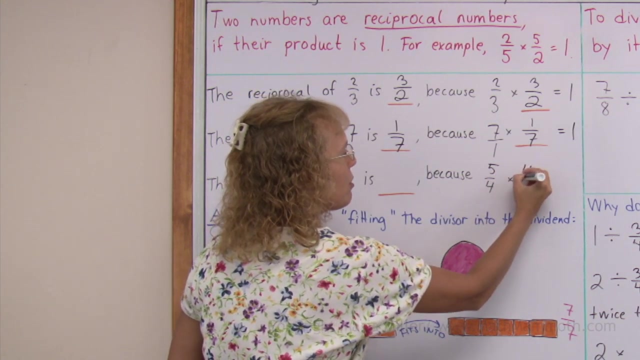 is one over seven. How about a mixed number, The reciprocal of one and one-fourth? Now, over here it helps. if you first write this mixed number as a fraction, It is five-fourths, right, And then five-fourths times four-fifths would equal one, because you get twenty divided by twenty. So we get 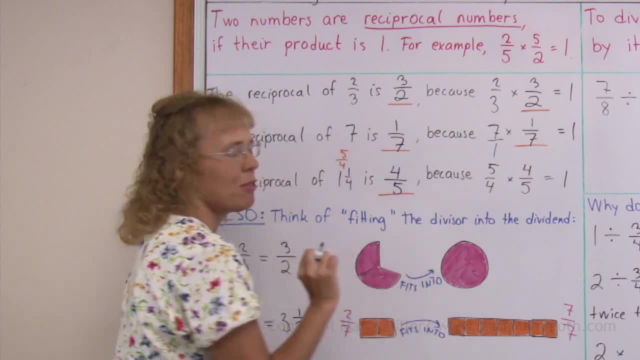 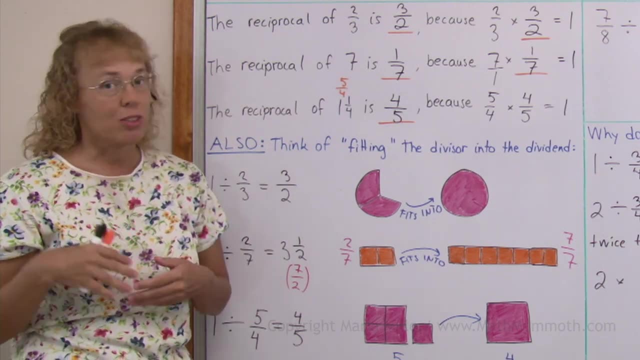 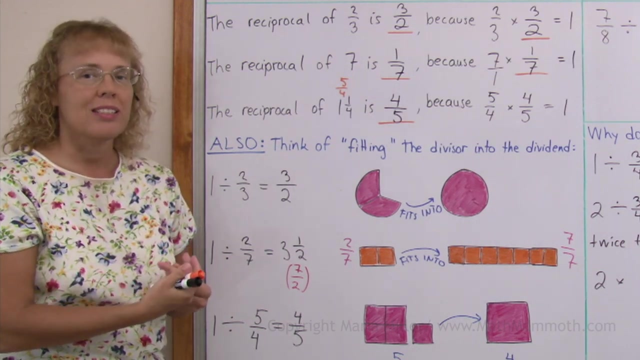 four-fifths. here Again, flipping it works, but you have to first write it as a fraction. Now I want to tie this with a certain meaning for division In any division problem. if you have whole numbers, for example, you can think of the division problem as fitting. 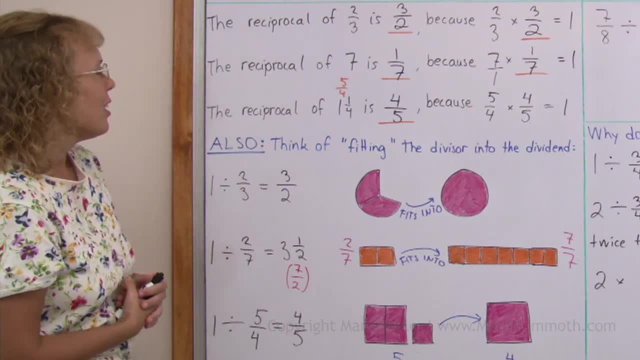 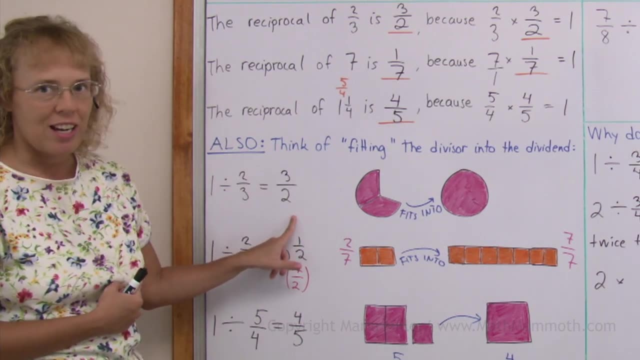 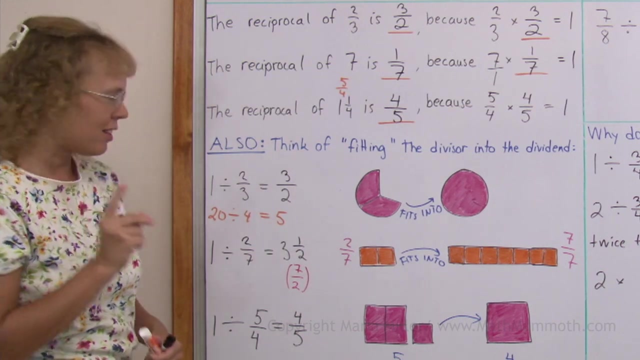 the divisor into the dividend, For example. this is a division problem, right? I could even have here: twenty divided by four equals five. Let me write it here for clarity. okay, In this division, you can think four-fifths into twenty, five times, right, Let's apply. 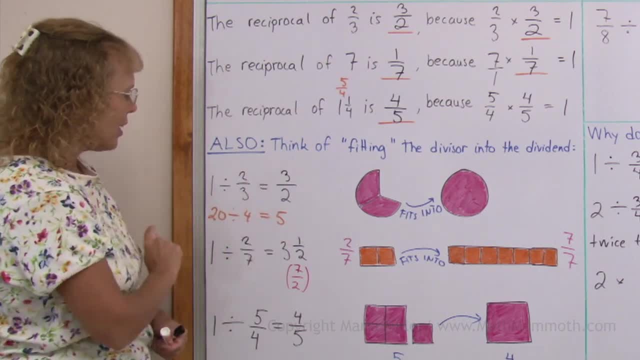 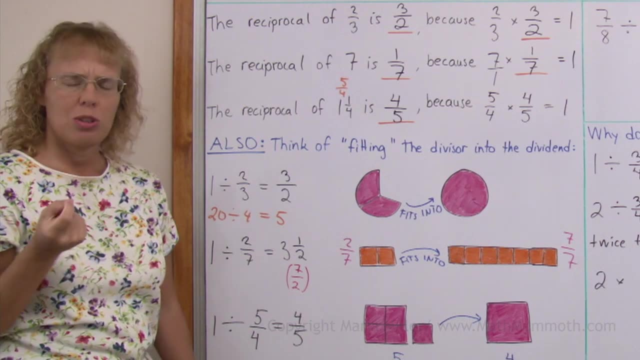 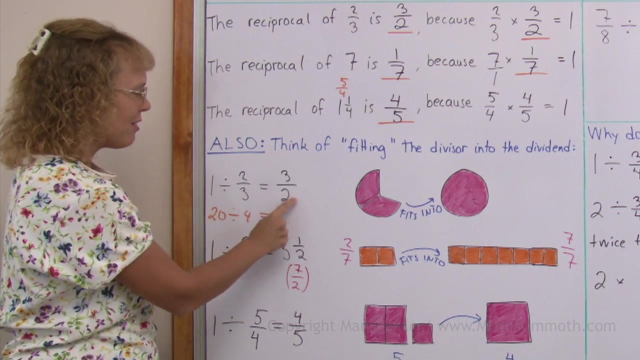 that idea. now to these fraction divisions. This division is one divided by two-thirds. okay, It equals three-halves. How do I know that? I know it because these two, when multiplied, give me one Three-halves times two-thirds. 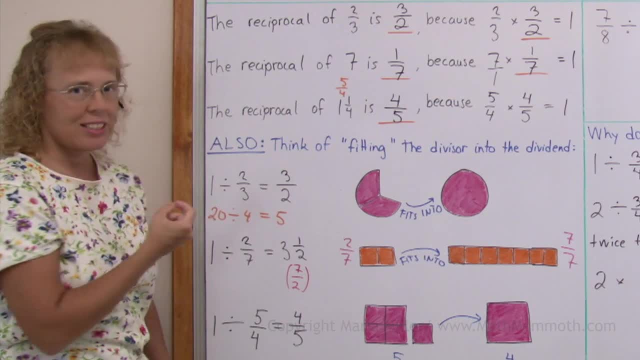 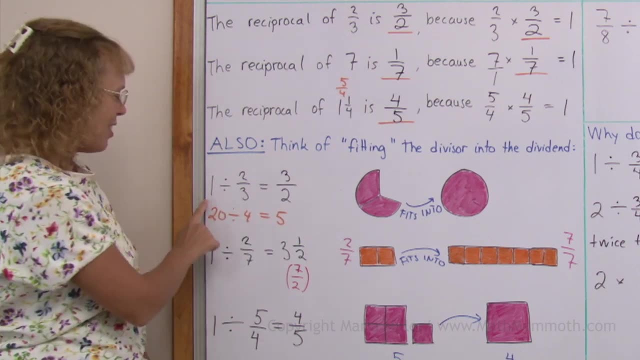 equals one. if I go backwards here, okay, We just studied that These two are reciprocal numbers, so when you multiply them you get one. So in division one divided by a fraction, the answer is: it's a reciprocal number. 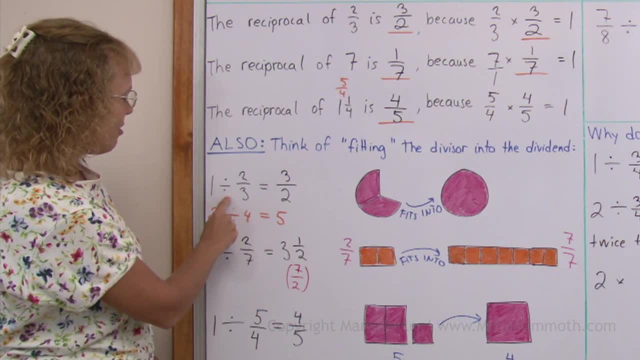 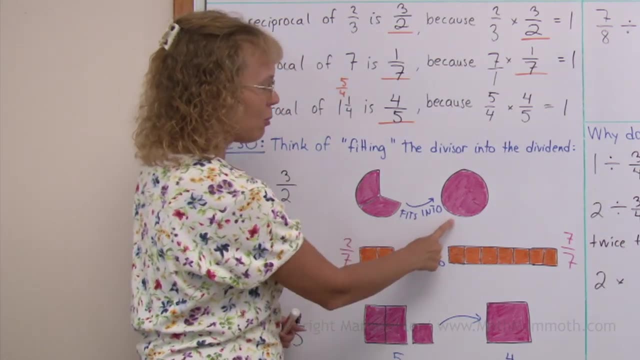 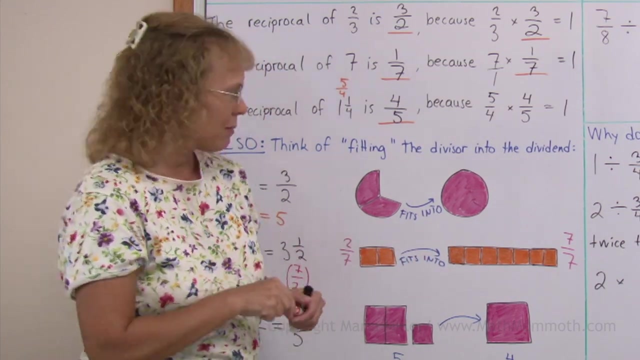 Now thinking of the fitting idea: two-thirds fits into one exactly this many times. Let's see: Here's two-thirds, Here's one. Does two-thirds really fit into one? three-halves or one-and-a-half times? Let me divide this into thirds. okay, Two-thirds fits right here, once right, And 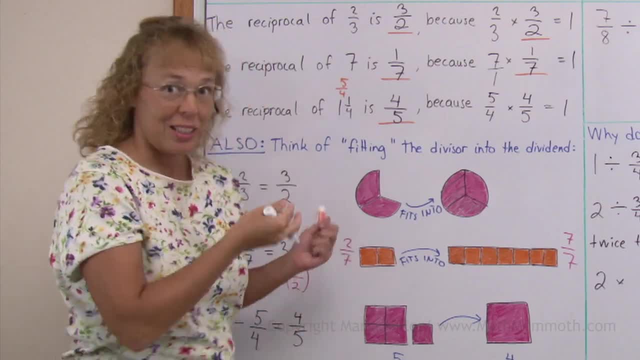 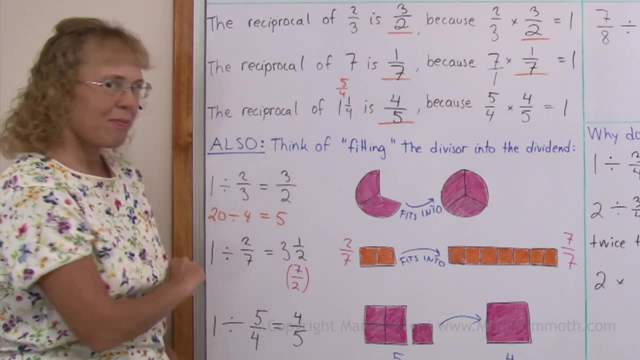 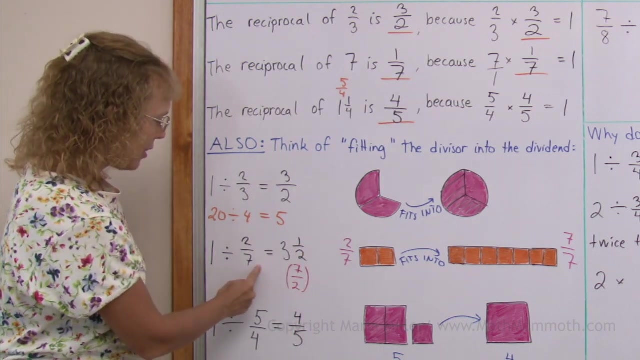 then also half of it fits over here. So one-and-a-half times, right? Let's look at this one, One divided by two-sevenths. Again, the answer is seven-halves or three-and-a-half, because if I multiply these, I get one. These: 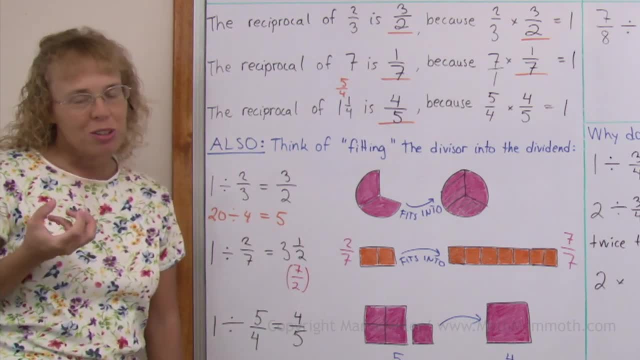 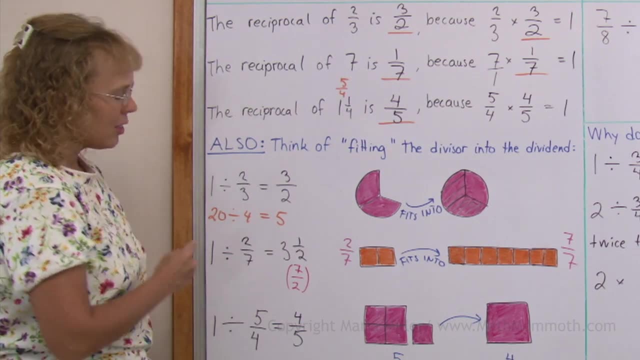 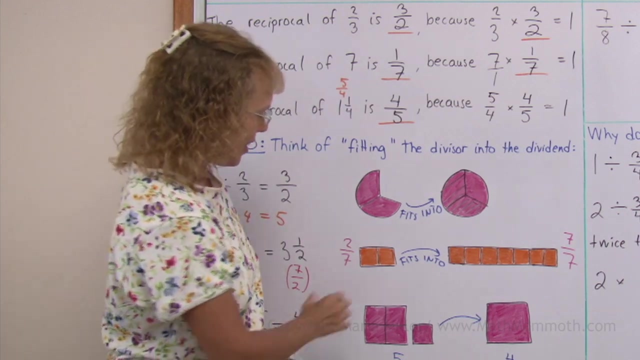 two are reciprocal numbers, But we can also illustrate it visually, thinking of how many times does this fit into this? So I have a picture here: Two-sevenths, one divided by two-sevenths, And then this is one-whole, or seven-sevenths. How many times does these? 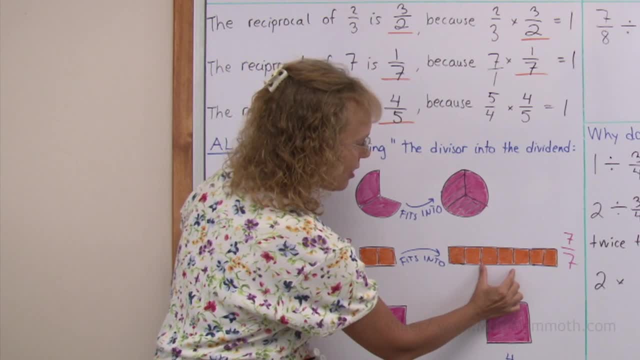 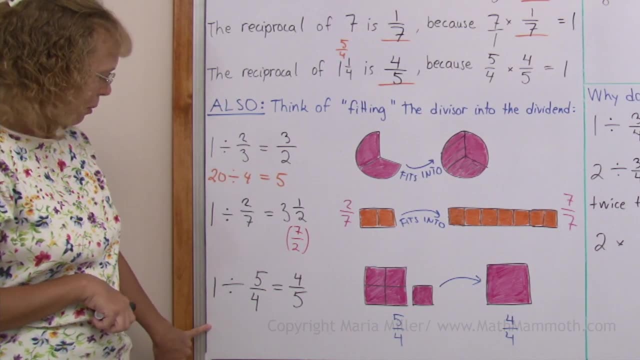 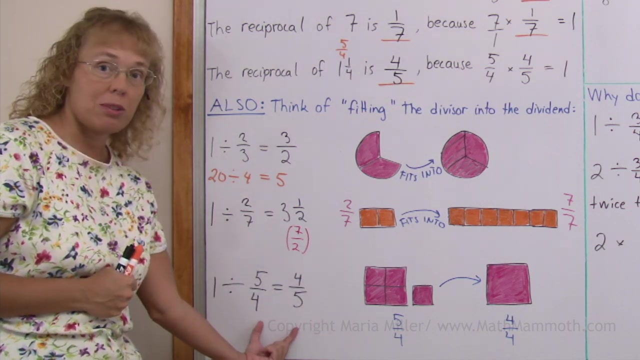 two-sevenths fit into here: Once here, second time, third time and half a time. right, Three-and-a-half times. Last one, One divided by five-fourths. Okay, I know the answer: It's four-fifths because these two are reciprocal numbers. If you multiply them, you get one. 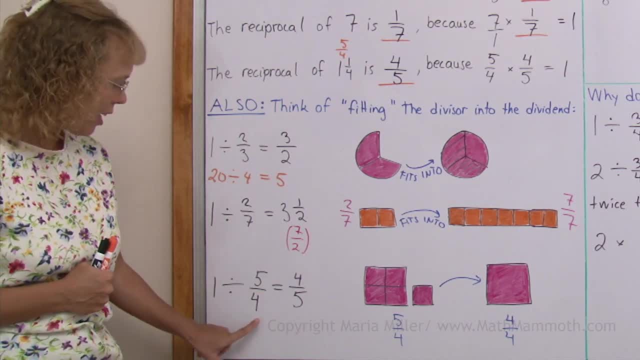 In the picture. I think: how many times does five-fourths fit into this? Okay, I know the answer: It's four-fifths, because these two are reciprocal numbers. If you multiply them, five-fourths fit into one. No, not even ones, of course. Here's my five-fourths. 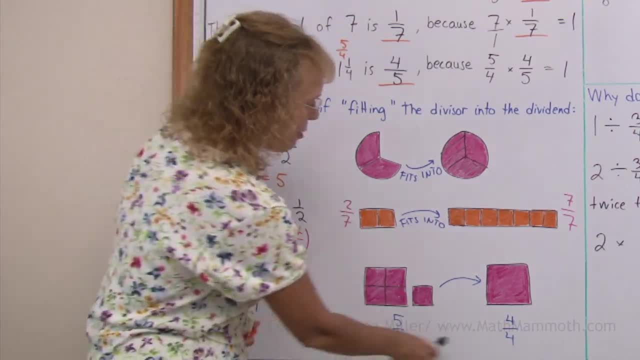 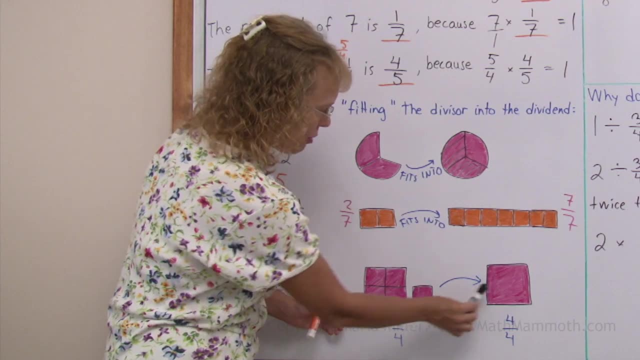 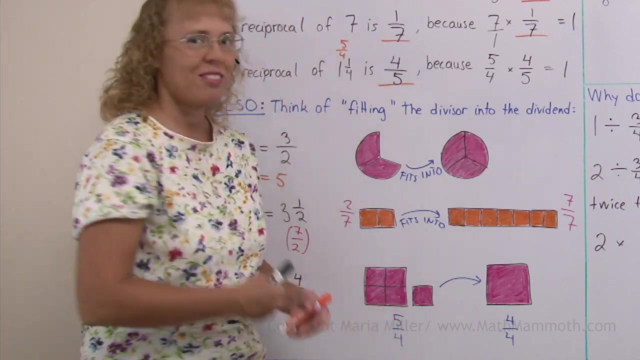 Here's my one, So it won't fit there, but a certain part of it fits there, right? You can think these four little parts would fit there, right, And these four little parts. if there's five parts, then these four little parts are four-fifths. 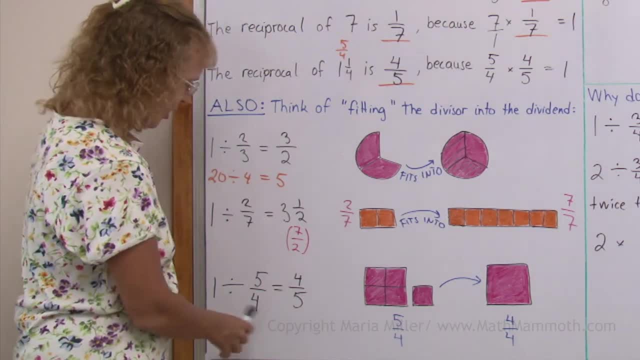 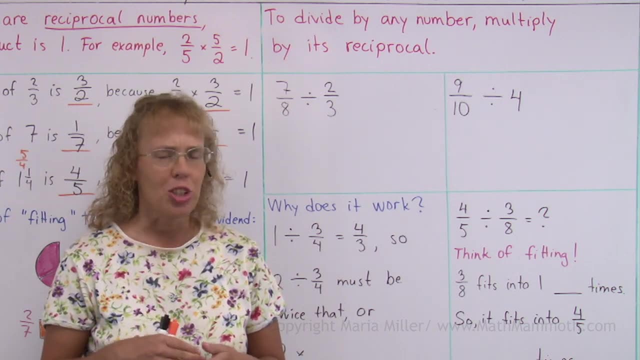 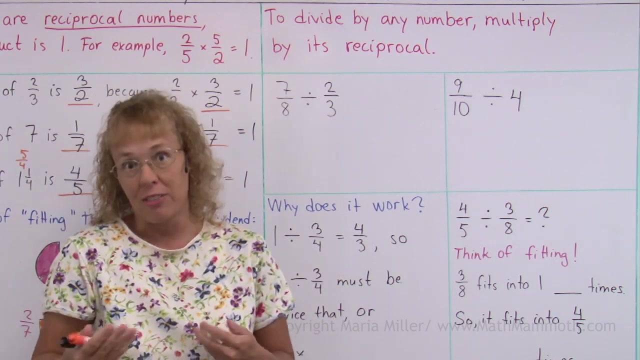 of this thing here, right? So four-fifths is the answer. Now that we have studied reciprocal numbers, we can go back to the shortcut for fraction division, And I wrote here- to divide by any number, for example, to divide by a fraction multiply. 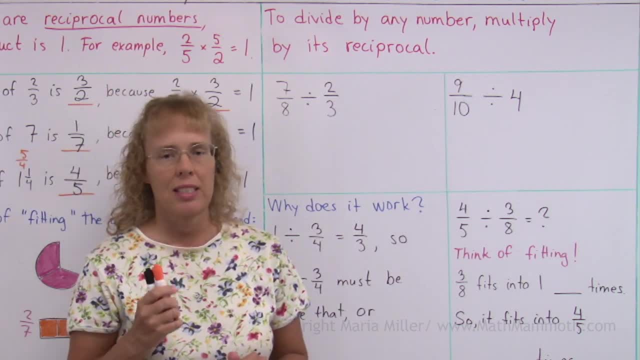 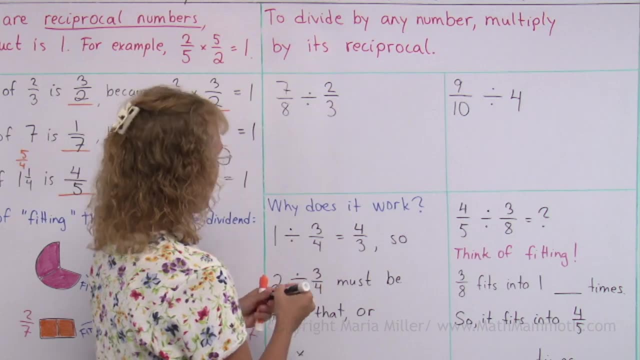 by its reciprocal. This means that we will change every division problem here into a multiplication problem. And this is how it happens. Subtitles by the Amaraorg community. I will write the seven-eighths. It won't change. The division changes into a. 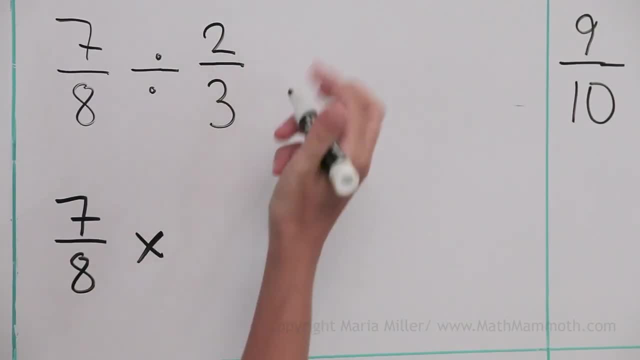 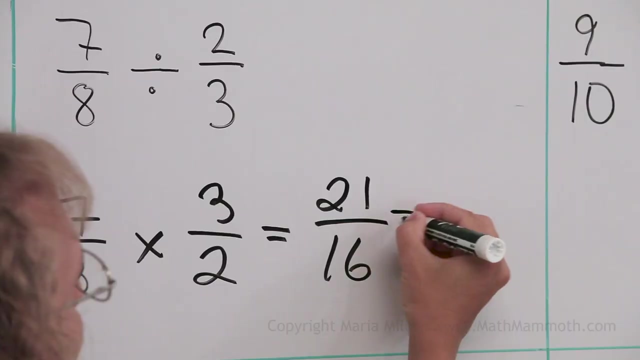 multiplication And then this number: I take its reciprocal, so I flip it like that, And now over here we just multiply: normally Seven times three is twenty-one and this is sixteen, And then lastly, write it as a mixed number: It's one whole, and 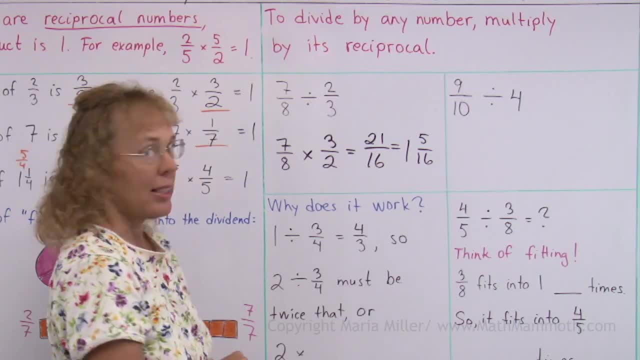 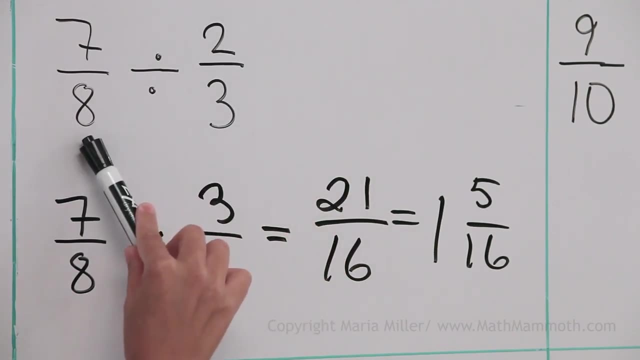 five, sixteenths. Does it make sense? You can think of it like this. You can write it like this. You can write it like this. You can think of the fitting Two-thirds fits into seven-eighths And over here, okay. 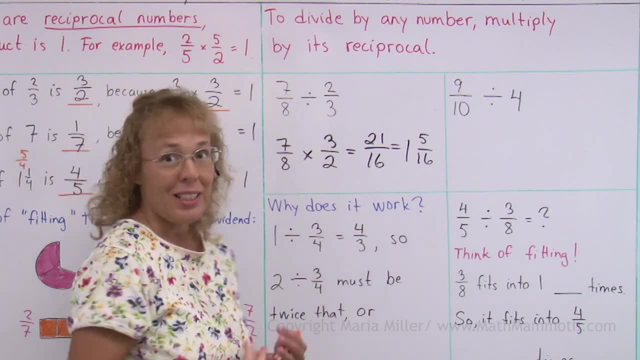 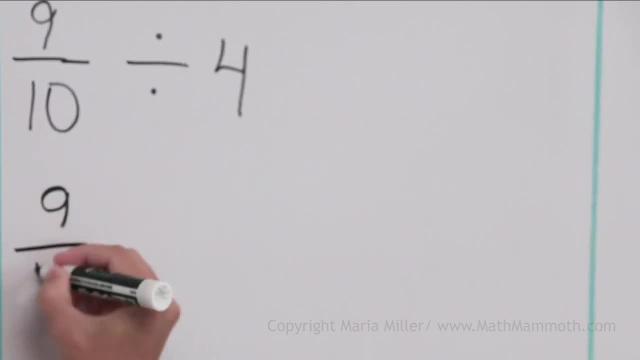 somewhat over one time. Yes, that makes sense. Nine-tenths divided by four. Okay, I do the same. This first fraction does not change. This changes into a multiplication. And now I write the reciprocal of four, which is one-fourth. 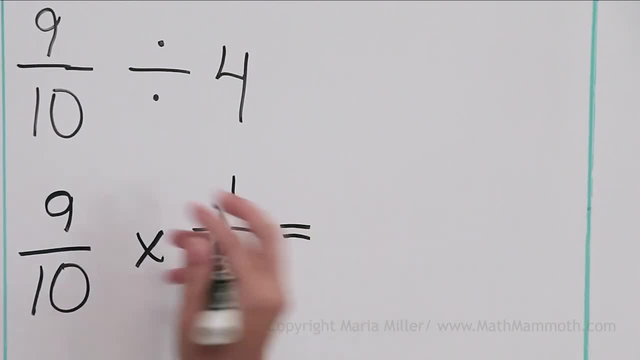 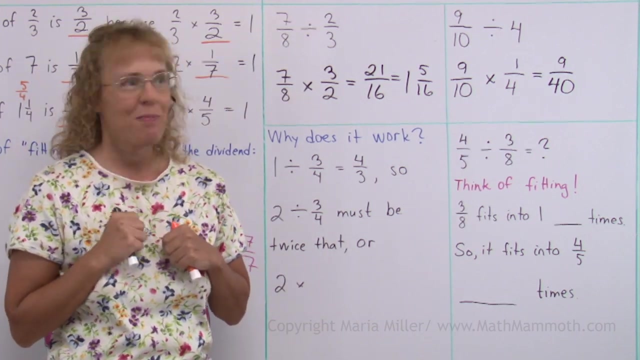 And then we multiply 9 times 1 and 10 times 4, which is then 9 over 40. Now we will spend just a little time trying to understand why this shortcut works. It is based on those reciprocal numbers and that fitting idea once again. 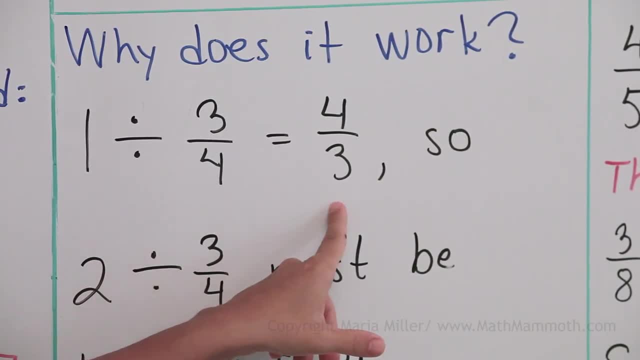 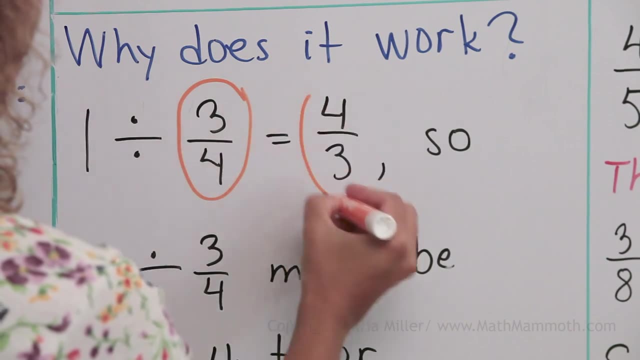 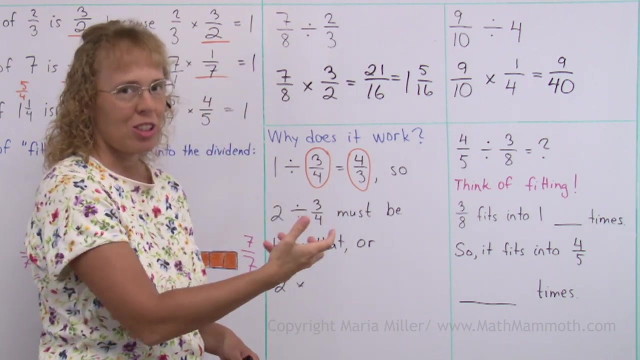 For example, 1 divided by 3 fourths equals 4 thirds. Now how do I know that? You should know it too? These two here are reciprocal numbers, so if you multiply them you get 1.. So that's where you get that division, because division is the opposite operation of multiplication. 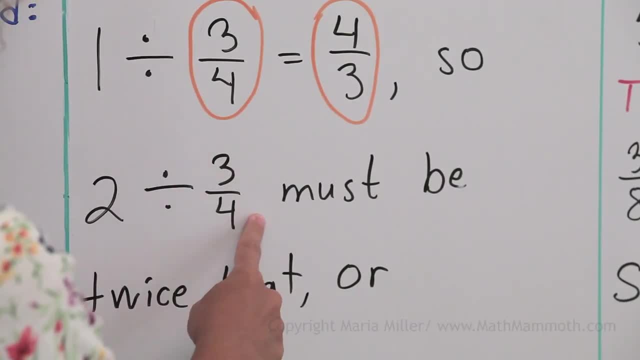 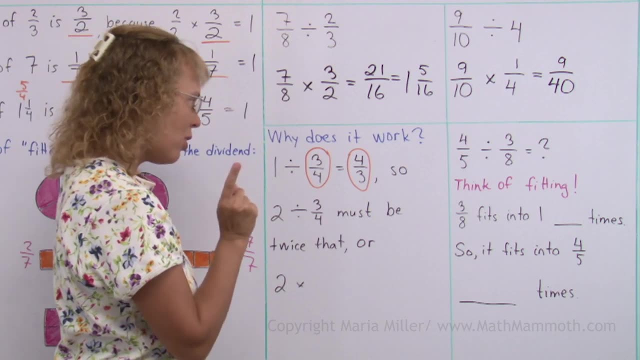 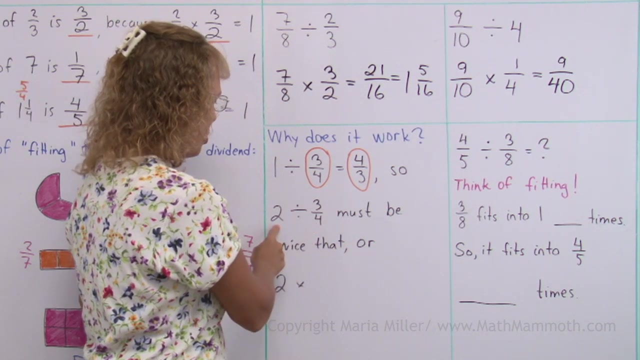 So then, if you have this kind of a division problem- 2 divided by 3 fourths- the answer to that must be double or twice the answer to this problem here, Because if 3 fourths fits into 1 that many times, then 3 fourths fits into 2.. 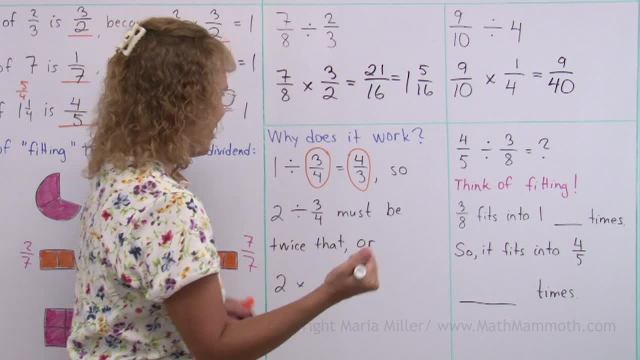 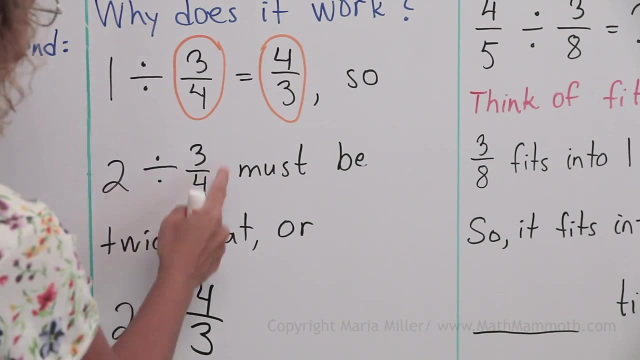 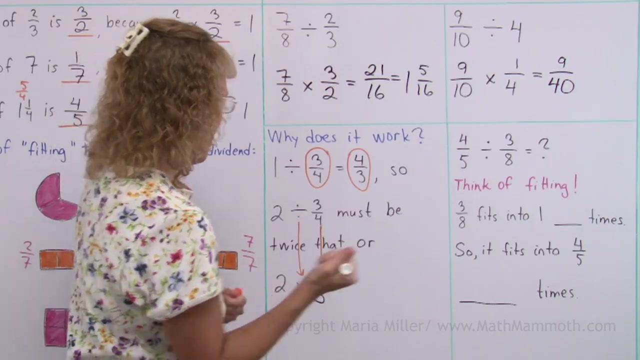 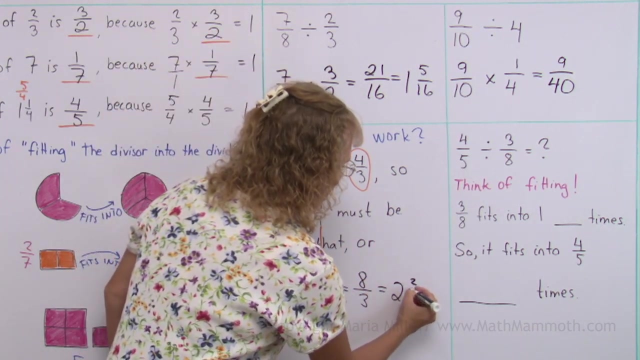 So twice, that many times right, Twice times 4 thirds. So now you see here, this division problem here has changed into a multiplication by these numbers, reciprocal, And then you would multiply 2 times 4 is 8, 8 thirds, which is 2 and 2 thirds. 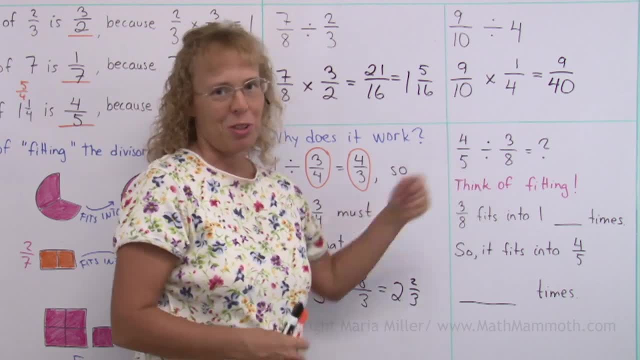 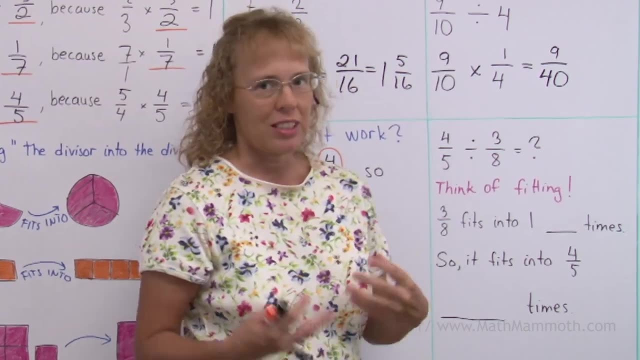 So this was an easier type of division. Let's try another That is more difficult: 4 fifths divided by 3 eighths. Okay, We'll think of this fitting. How many times does 3 eighths fit into 4 fifths? 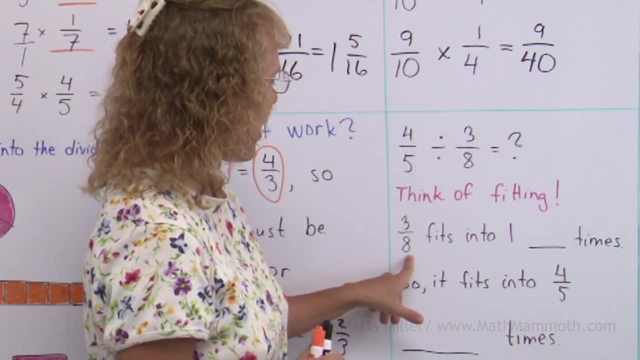 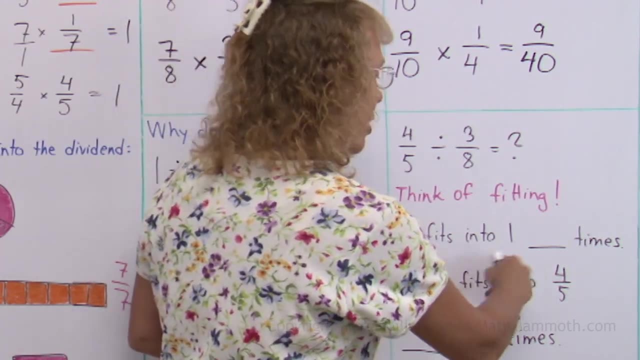 We don't know. But we do know how many times 3 eighths fits into 1. From the reciprocal numbers we know that right 3 eighths fits into one whole exactly 8 over 3, 8 thirds times. 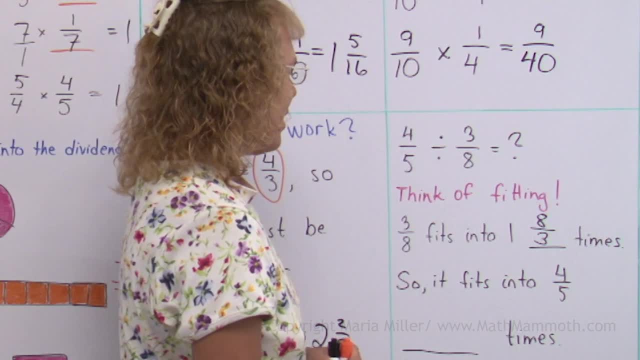 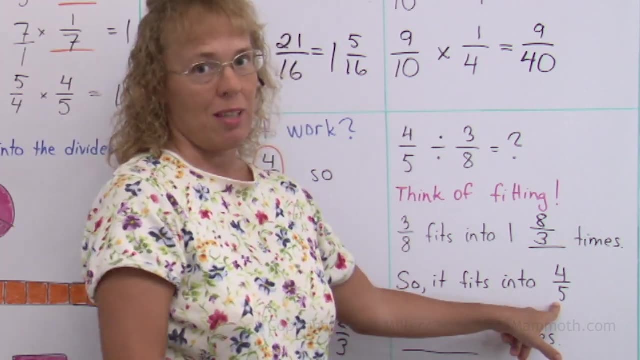 Or that is 2 and 2 thirds. So 3 eighths fits into 4 fifths, 4 fifths. that many times- I hope you can follow that reasoning- 3 eighths fits into 1. that many times.